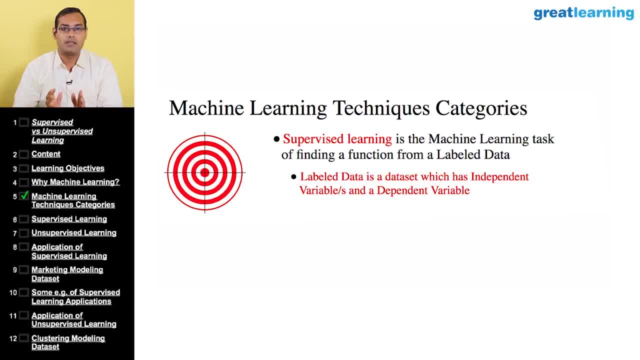 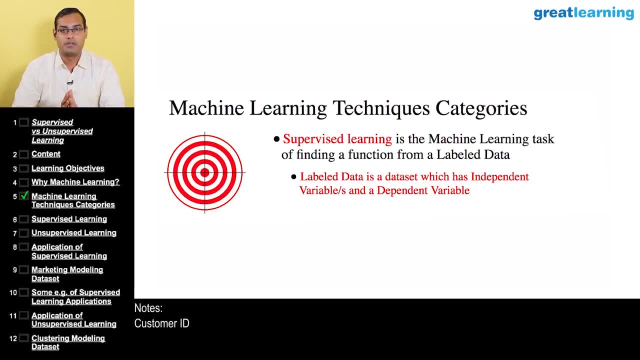 I have got a data set which has got many attributes, many variables. For example, I have got data of my customers: customer ID, age, gender, occupation, their transaction behavioral attributes And I have one more additional information saying whether the customer has churned or not churned. 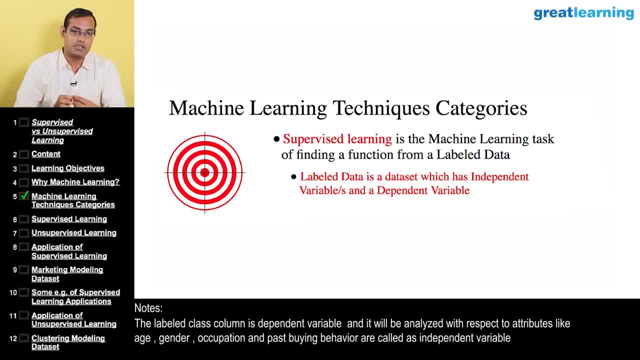 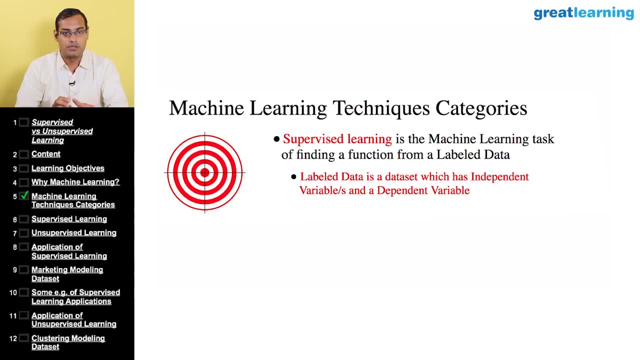 This column which says which customer has churned and which customer has not churned, is called the labeled data. This kind of data when I analyze to understand the profile of customers who have churned vis-a-vis the profile of customers who have not churned. 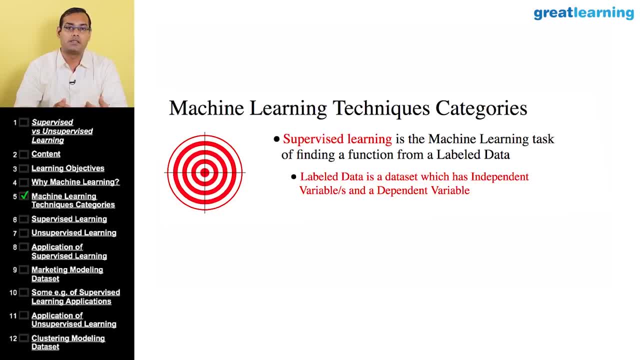 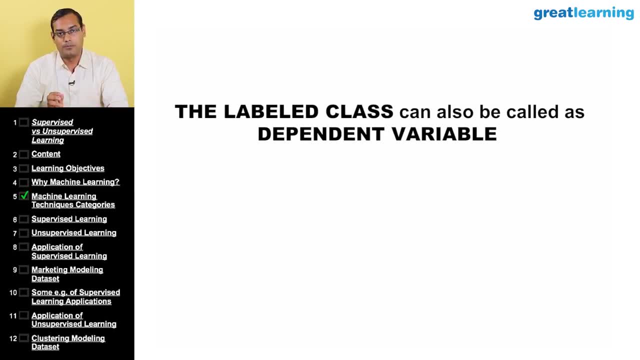 I use a technique which will fall under the head: supervised learning. The labeled class column can also be called as your dependent variable. And these classes when I analyze with respect to variables like age, gender, occupation and their past buying behavior, Those variables are called. 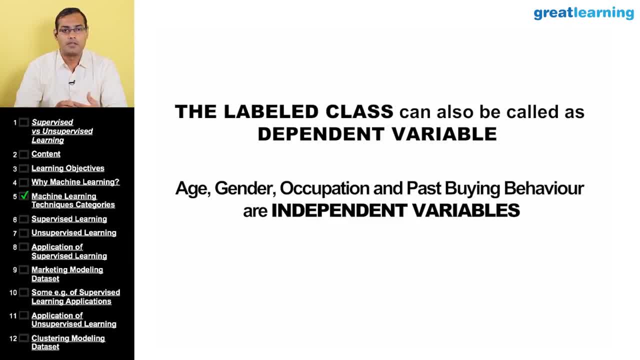 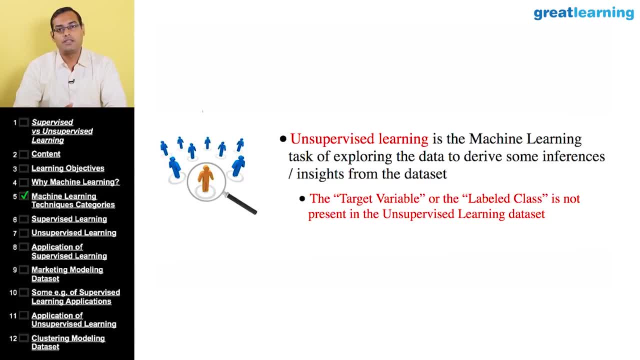 independents variables. Let's now see what is unsupervised learning. Unsupervised learning is a machine learning task of exploring the data to derive some inferences or insight from a data- The same data which we talked about, where I had data of my customers: age, gender, occupation and a class which is whether 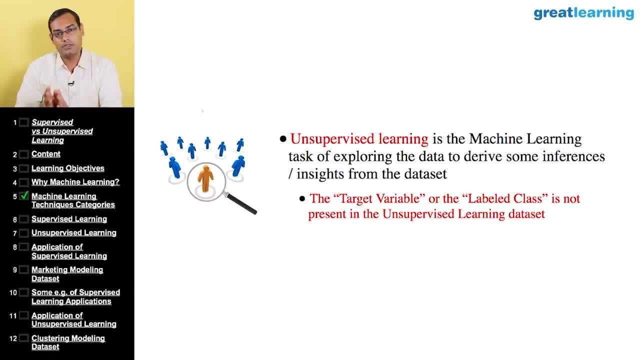 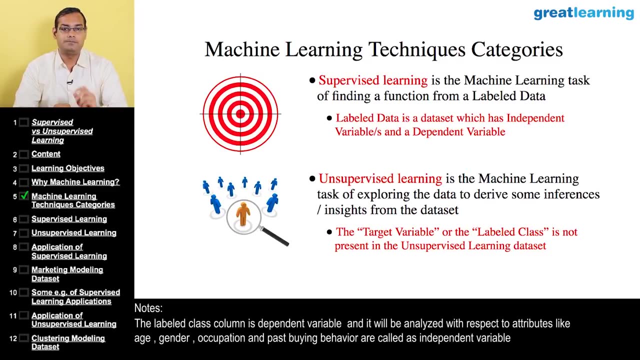 the customer has churned or not churned. If I remove this column, I assume that this column, whether the customer has churned or not churned. if that column is not present in my data set and if I analyze the data in that case, this: 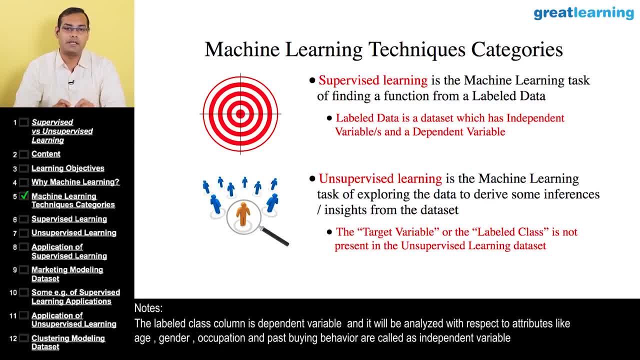 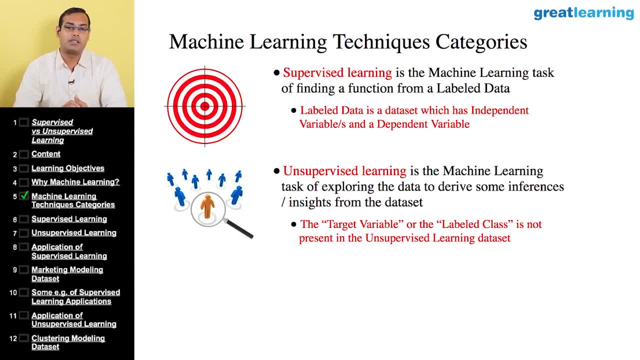 analysis will form the data. This analysis will fall under the head unsupervised learning. So in unsupervised learning, I would be doing analysis to find out what are the different types of customer segments that I have, or what are the types of attributes which are. 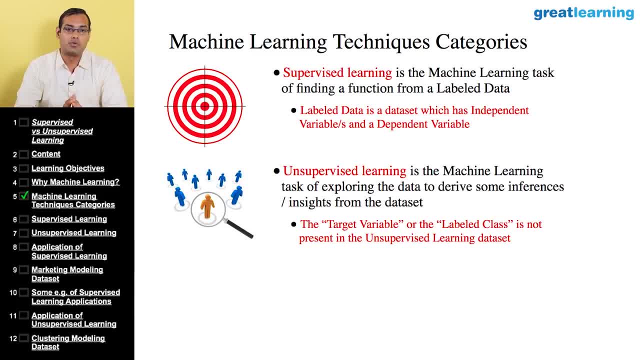 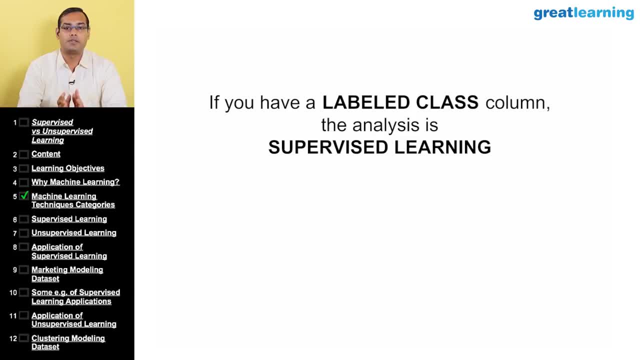 similar between various customers. All those things would go under the head of unsupervised learning. So, broadly speaking, if you have a target variable or a labeled class column and then you are doing an analysis, in that case it will be a supervised learning. If you do not have a labeled, 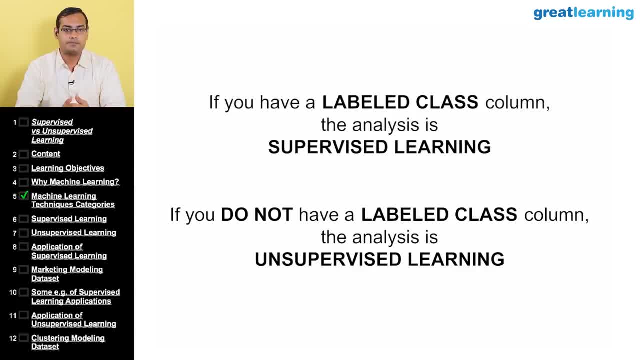 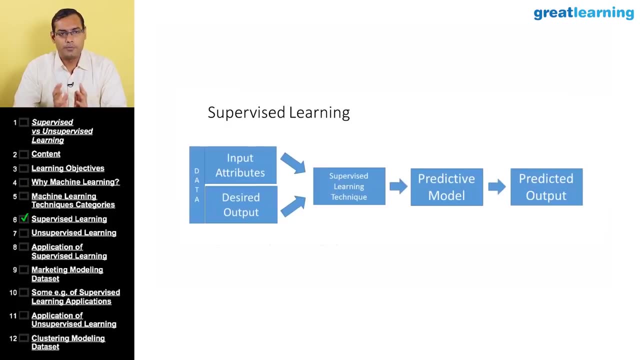 class column and you are doing analysis, it will go under the head unsupervised learning. Let us now try to understand supervised learning in slightly greater length. In supervised learning, when you have a data set, there will be input attributes called independent variables, and there will be a labeled class column which is: 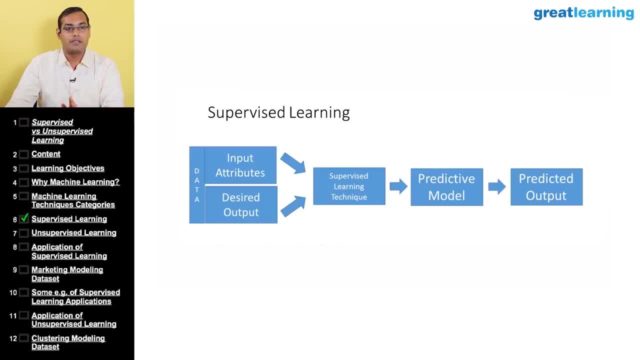 your target variable or the desired output. Now you are trying to analyze the data wherein you are trying to establish a relationship between your labeled class and your target class. There will be an independent and an independent input variables, feature variables. So to analyze this, you pass this data set through a learning algorithm which 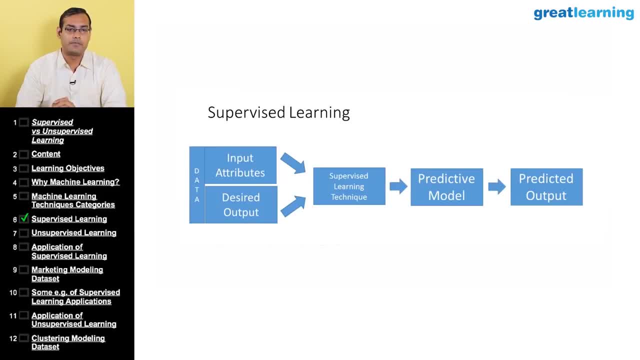 will be a supervised learning algorithm. The supervised learning algorithm will try to find patterns and relationship between the input attributes- Independent variables, when they match with theAm fiquei, st, Кол masih là, ph strand variables- and the dependent labelled class, Based upon the relationships it identifies. 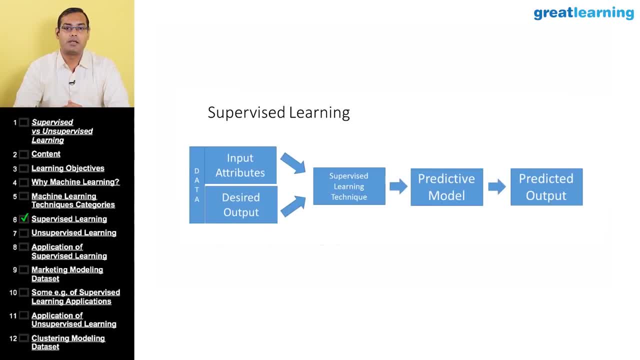 it is going to give you a model and that model we call a predictive model And, based on the predictive model, it is also going to predict the output of those set of records, And this is called a supervised learning process. To check the model performance, what we can do is 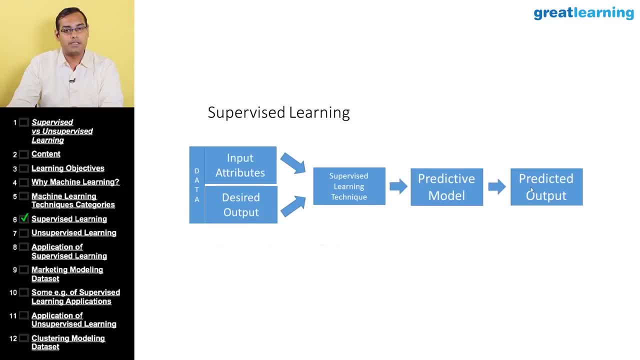 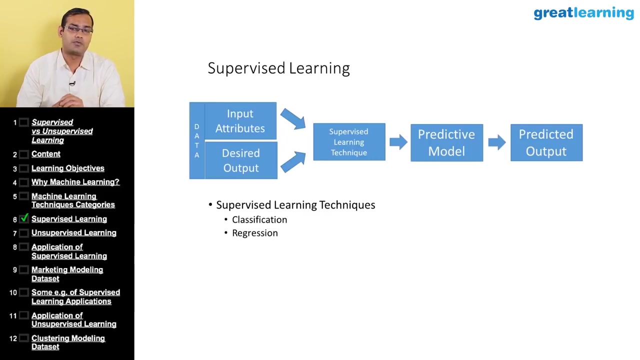 we can compare the output which is predicted with respect to our desired output And, based upon how accurate we make prediction, we can have various model performance measures. This is what a supervised learning algorithm is all about. Two main examples of classifications of supervised learning techniques. One is a classification and second 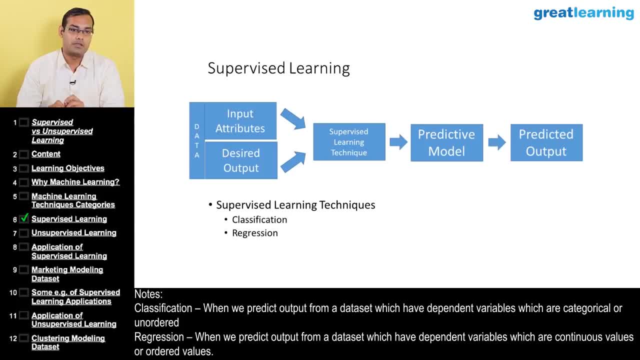 is regression. Classification comes when, when we are trying to predict the output, which is, say, class A versus class B, When the output prediction is about a class, which record will fall under which head? I will find one variable which is aboutizin the output, For example credit card intersection. I want 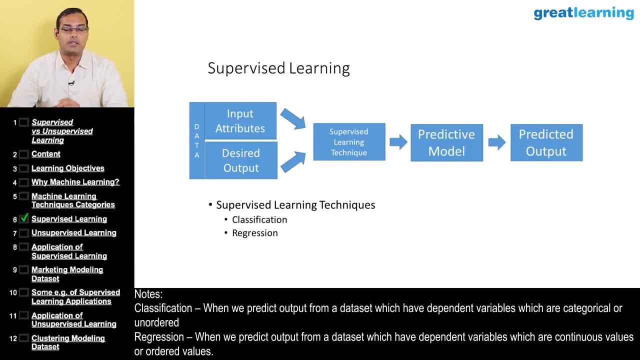 to predict whether a credit card intersection is a fraudulent transaction or a not fraudulent transaction. In that case it comes a classification problem: Regression, When my target value is a continuous variable. For example, I want to predict the amount a customer is going to give or the value of the management support which is now going to be A and A plus. So a configuration is going to tell us and 있는 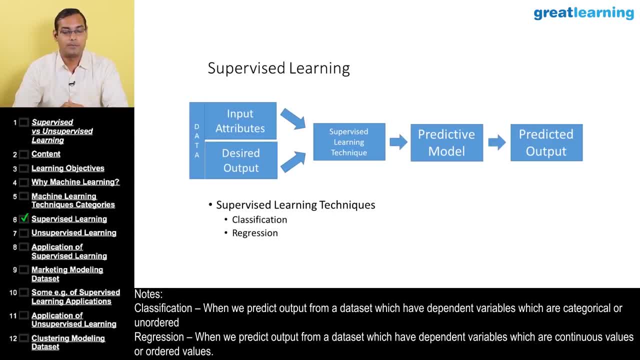 to spend on a credit card. based upon his past purchase patterns and if I'm trying to make a prediction about the spends the customer is going to make in the next month, it will be a continuous target variable. in that case we will call it as a regression process, So supervised learning. 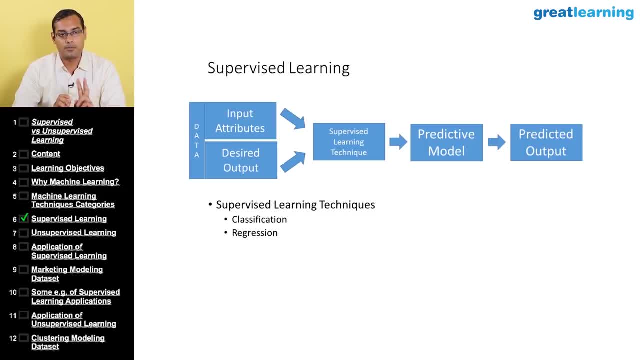 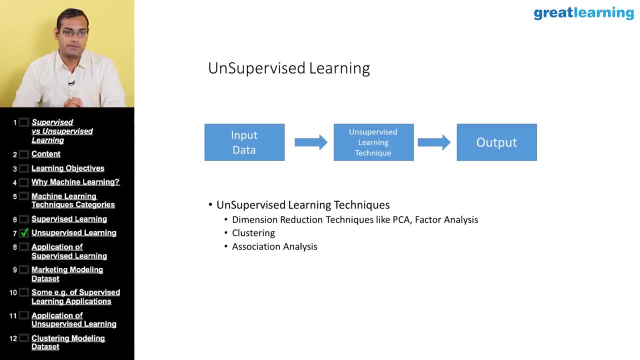 techniques to main broad classifications, to broad class categorization. supervised learning techniques are classification or a regression technique. Now let us come to unsupervised learning technique. In an unsupervised learning technique, as I already mentioned, we do not have a labeled class. we have a input data and we are trying to 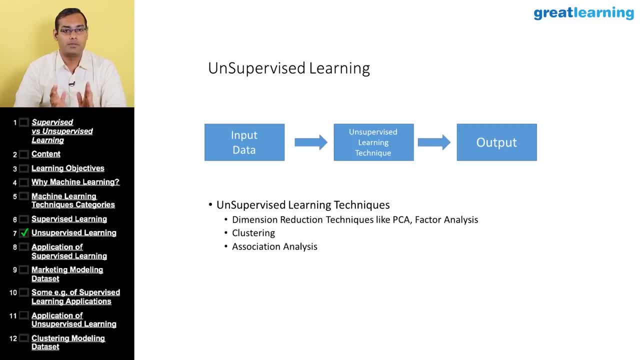 analyze things with respect to the given set of input data and this set of data when we analyze using some unsupervised learning technique. there are three main classifications. one is called a dimension reduction technique. For example, when I have got data and I'm trying to reduce the number, 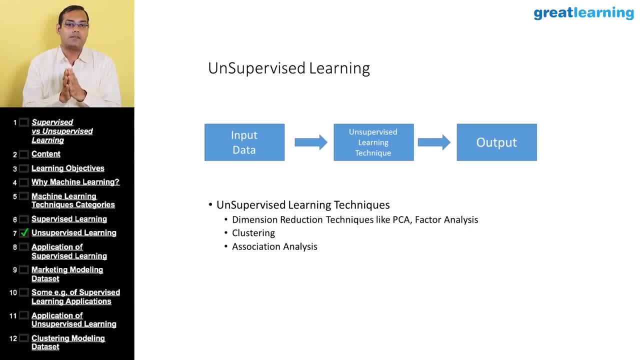 of variables in data. in that case, I call it as a dimension reduction technique. Some of the dimension reduction techniques most used are: principal component analysis, factor analysis. Now, when the same data, when I'm trying to reduce the number of records, number of cases, that supervised learning technique, unsupervised learning technique. 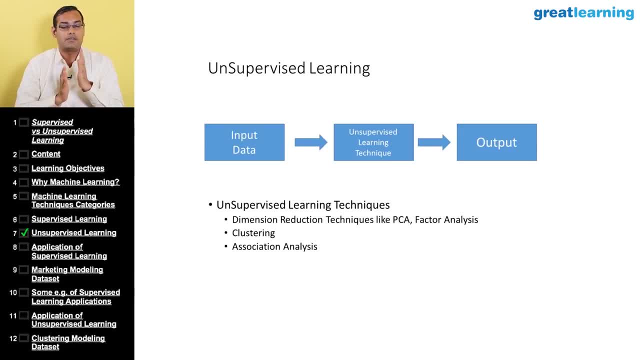 we call clustering. and there is a third type of unsupervised learning technique which is called association analysis. example: market basket analysis. In a market basket analysis, what we try to see? what are the different products, what are the different items the customer buys together? 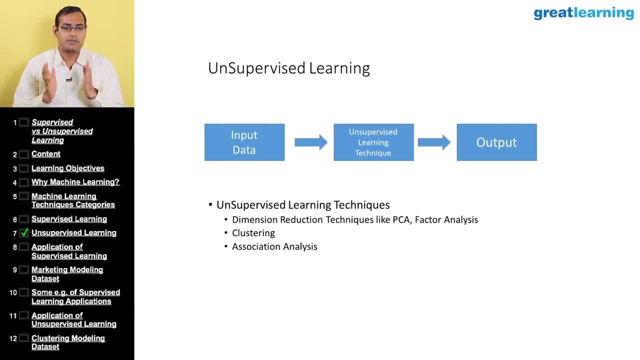 This kind of association analysis is very commonly used by e-commerce for recommendation engine. You buy up certain product on an e-commerce portal and the website automatically suggests you what is the associated product that many other consumers have purchased along with it. that is called association analysis in unsupervised learning technique. we 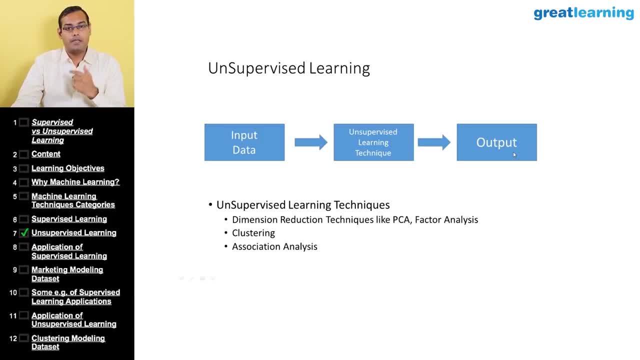 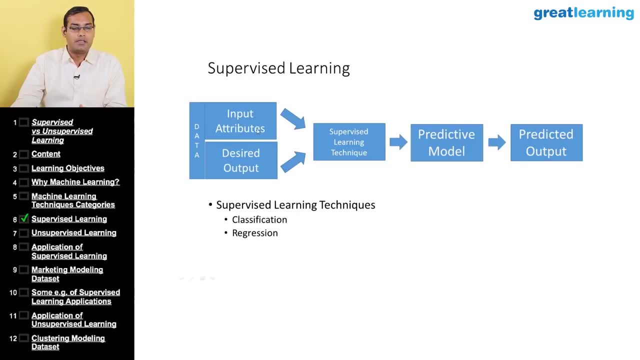 directly get a output. if you compare a supervised learning versus unsupervised learning, let's go back to a supervised learning slide. in a unsupervised learning, you see we had an input attributes and we had desired label class. the algorithm tries to find a relationship between the target variable. 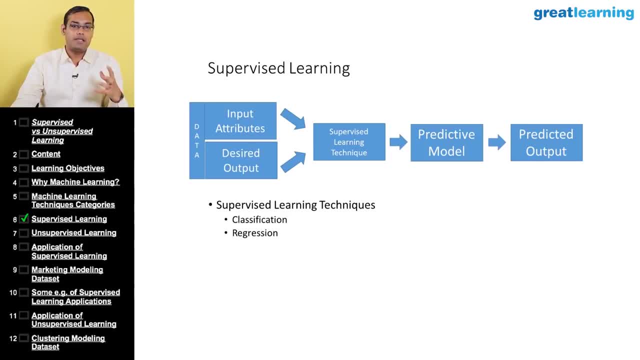 and independent variables and based upon that, it builds a model which is a predictive model and you get a predicted output. I can save this predictive model and I can use this predictive model for future prediction about new set of records that I get for these new set of.